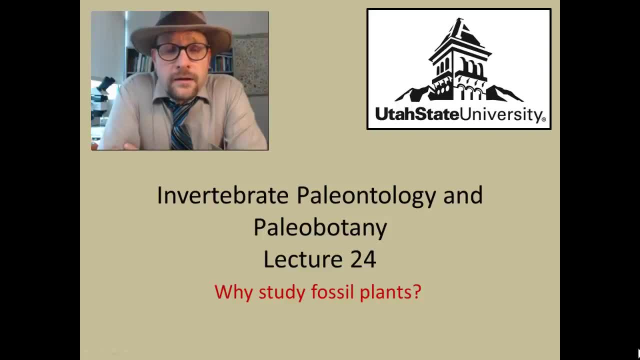 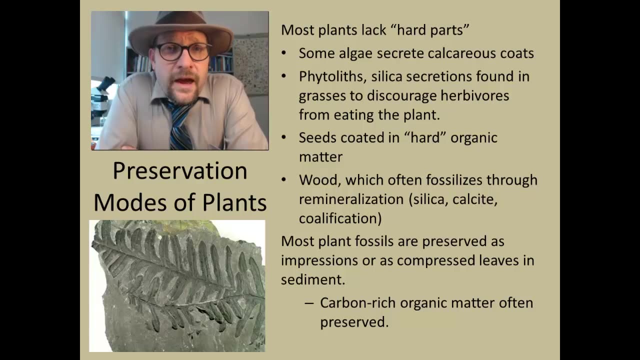 Hello and welcome to Invertebrate Paleontology and Paleobotany at Utah State University. This is lecture 24, in which we will answer the question: why study fossil plants? Unlike the invertebrate animals we have been looking at in this course, most plants lack. 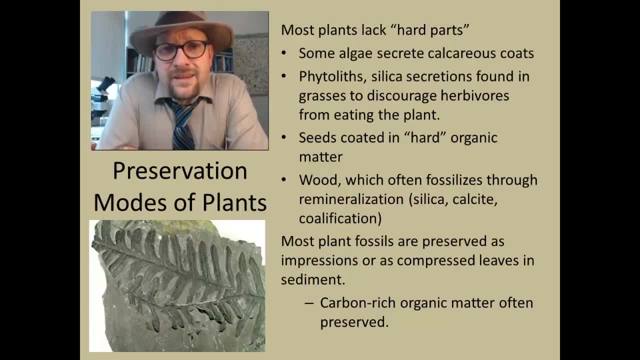 hard parts. A few plants and parts of plants can be fairly hard and in that case they can be preserved in the rock record more than other parts of the plant. For example, some algaes secrete calcium carbonate coats, and we will talk about some of the different types. 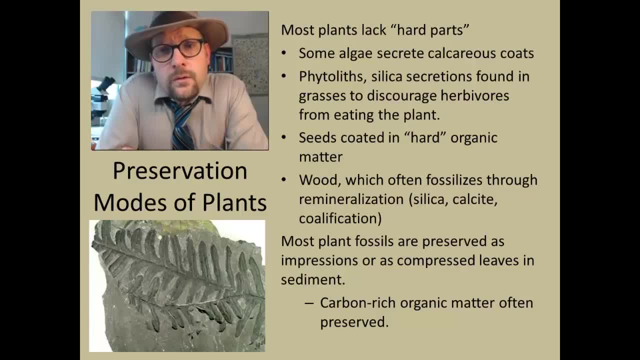 of algae or protists that can be preserved either through calcareous coats or even silica in the case of diatoms and flagellates. We also can have silica that is secreted by many plants and produce what are called phytoliths. We will talk more about phytoliths later on. 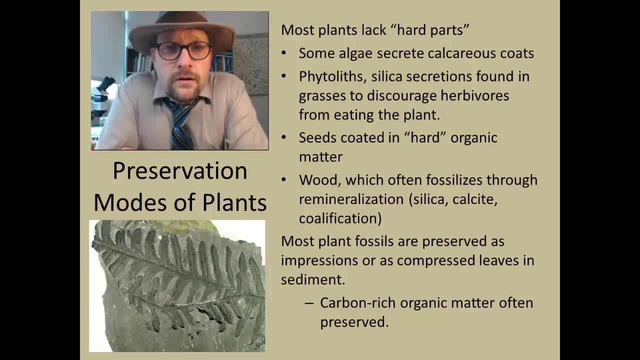 this semester. Those are hard parts that can be preserved in the rock record as well. Seeds themselves tend to be a very hard part, and so when we talk about seed plants, some of those can actually have a calcareous skeleton to them, or a hard part to them, and so they. 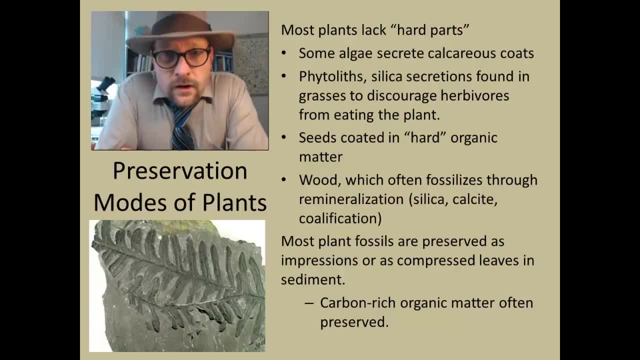 can be preserved. Wood which is very hard and we use it as a building material, is often preserved. What is interesting about fossil wood- petrified wood- is that it is often a replacement of silica or calcium carbonate into the original organic matter that composed 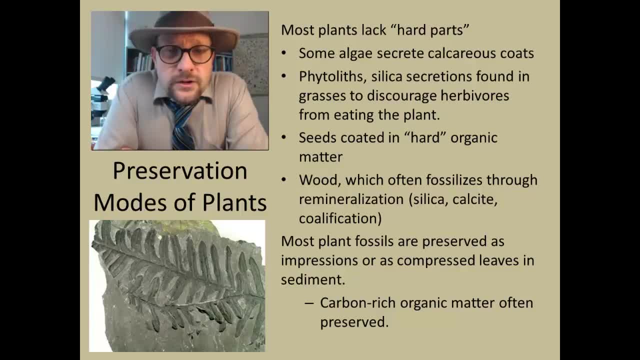 the wood, Although there is another process of coalification that is, under heat and pressure, changing the wood into smaller chains of hydrogen and carbon. Those polymers become smaller and they get compressed and that is the process of coalification and that occurs with heat and pressure. 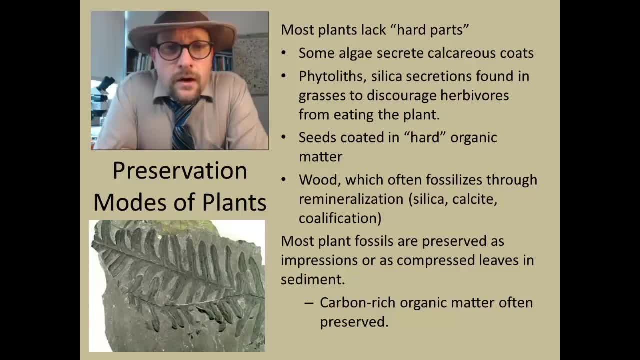 So often times you can get the formation of coal, petrified siliceous fossil wood or a calcite petrified wood. Most fossil leaves are preserved as either impressions of the leaf- so this is kind of like a mold and cast that you can get sometimes- or they are compressed organic matter. so 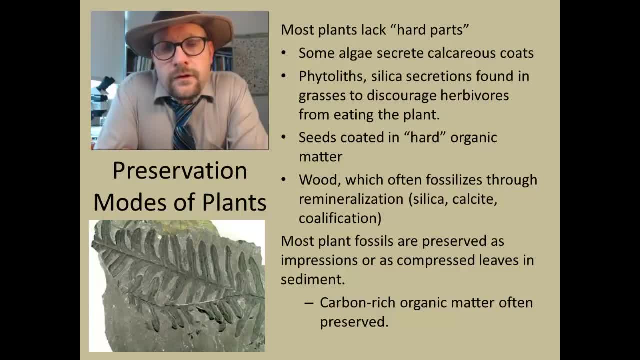 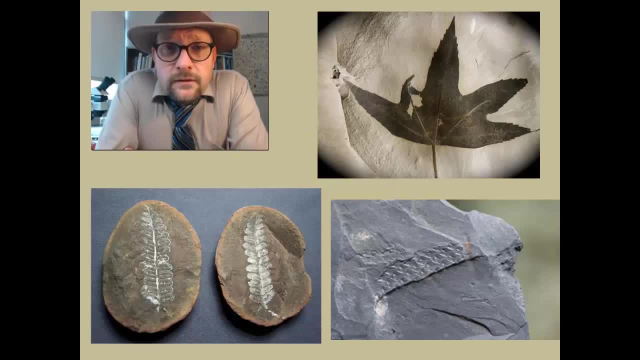 these are carbon rich organic matter that is preserved on the surface of most of the soil. Most fossil plants are very plentiful in terrestrial systems, and one of the nice things about terrestrial plants is that they give us a good indication of what the environment was like in earth's 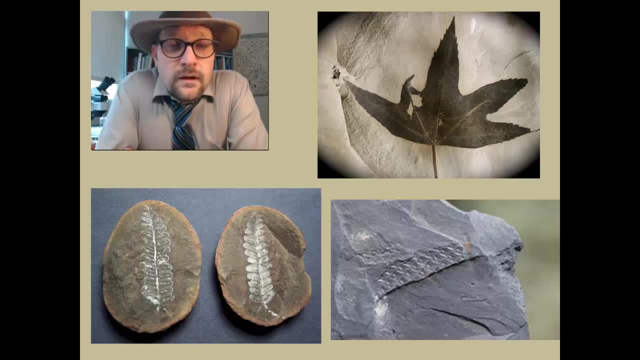 history on land, and so they give us a good insight into the types of plants that were living there and give us insight into the ecosystems of the terrestrial realm. That is one of the reasons I like focusing on fossil plants. One of the reasons I like focusing on paleobotany with this course is it is really important. 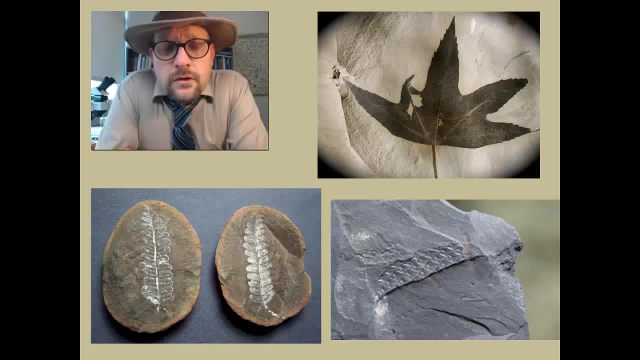 to be able to read the rocks in terms of looking at the terrestrial ecosystems, although many of the groups we will discuss in this class are also found in marine systems, such as the protists and the algaes, and some of the photosynthesizing organisms that live in the oceans today. 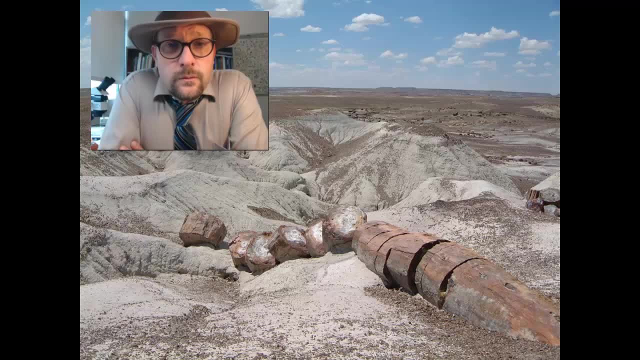 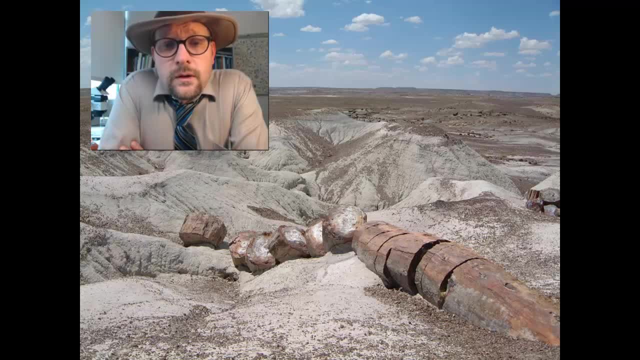 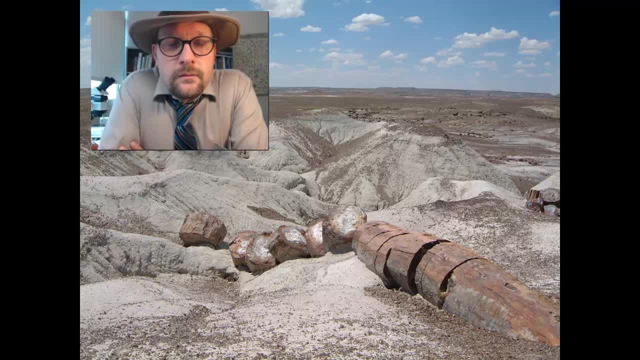 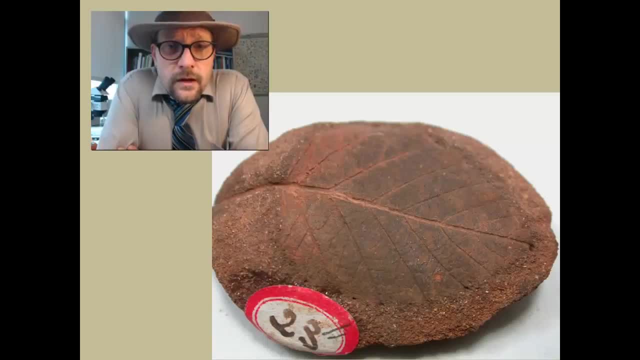 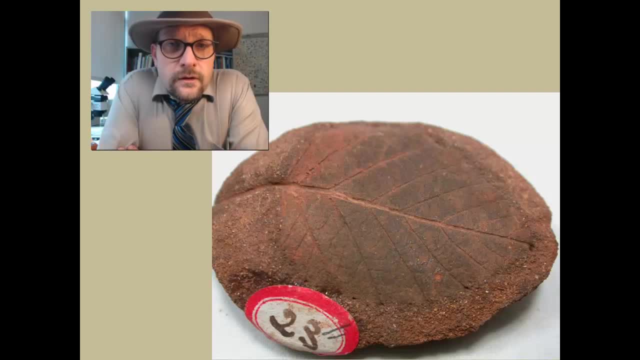 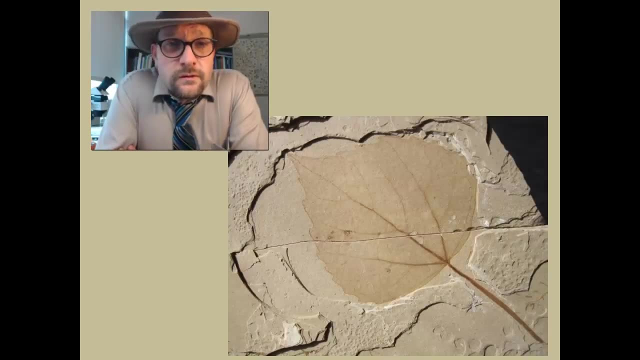 features, And so enough of the morphology of this fossil leaf is preserved that we can actually identify it. It's often times in shales in which you get the best preservation of fossil leaves, So this is a shale from the Florissant Fossil Beds in Colorado, where you get this wonderful. 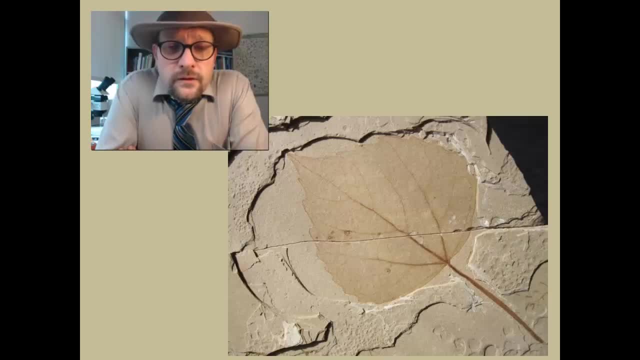 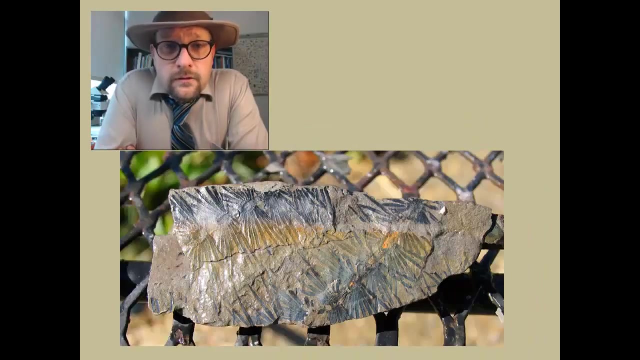 breakage pattern and you get this wonderful leaf pattern, And so these leaves can be very detailed and intricate in terms of their preservation and we can tell a great deal. We can even tell what types of insects were feeding on these leaves as well. Now we have a record of fossil leaves going back into some of the earliest of the land. 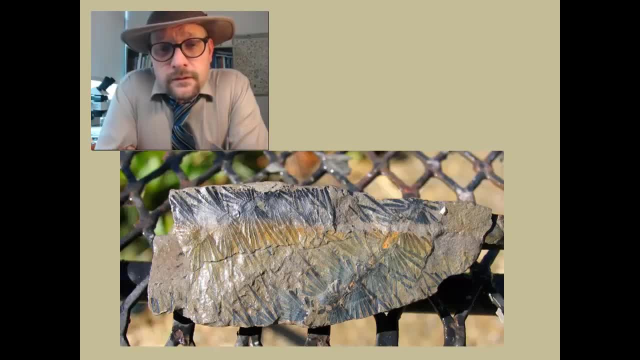 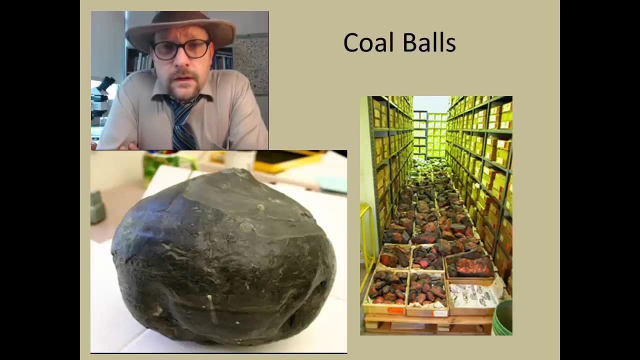 plants. This is an example of a Carboniferous Fossil from Pennsylvania. Some pretty exciting stuff that you can find, and we can trace the evolution of plants through many of these fossils. Now, fossil plants don't necessarily need to be impressions of leaves or fossil leaves. 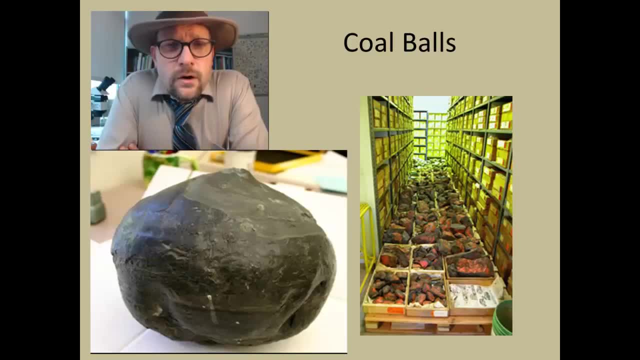 or petrified wood. They can be other things as well. These are what are called coal balls, and these occur in Appalachia, where you get these limestones. This is a limestone that is embedded within a coal bed, and these can actually preserve. 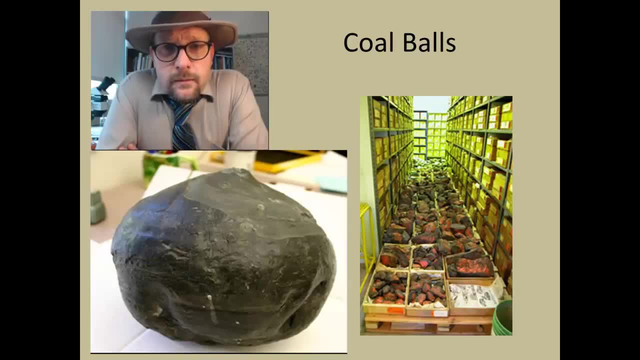 many times different components of the plant or the plants that were living at the time. So these are called coal balls. Now, fossil plants don't necessarily need to be impressions of leaves or fossil leaves or petrified wood. They can actually preserve many times different components of the plant or the plants that were living at the time in the forest in these coal balls. 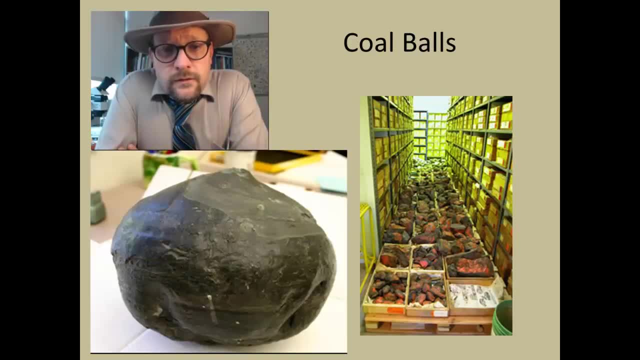 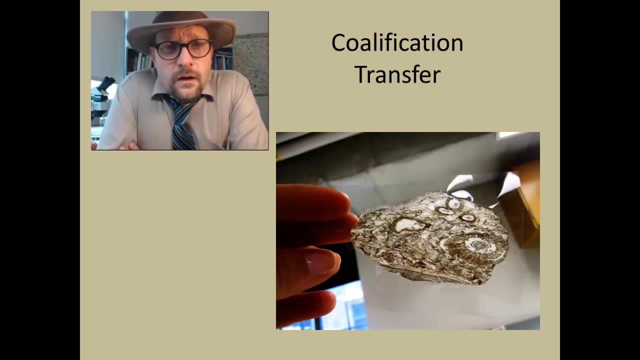 So they are often times studied, either dissolved out of some of the calcium carbonate to get the organic matter as well in these coal balls, or actually studied underneath a microscope to try to understand some of the plants that are actually contained in these things, Because what is often preserved with plants is actually the organic matter. you can actually 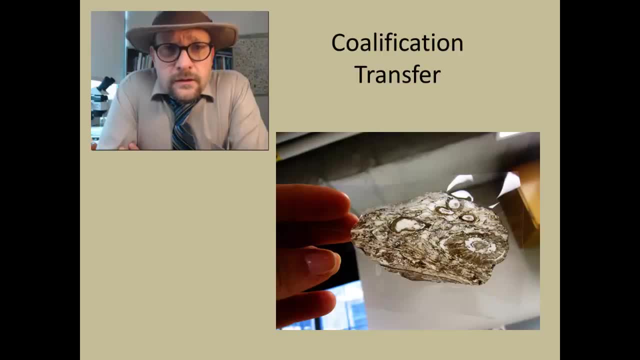 one of the things that many people do is using a variety of different acids, they try to etch away the surrounding matrix and to hold together that organic matter so it doesn't fall apart. often times paleobotanists will use sheets of acetate or some sort of plastic that they 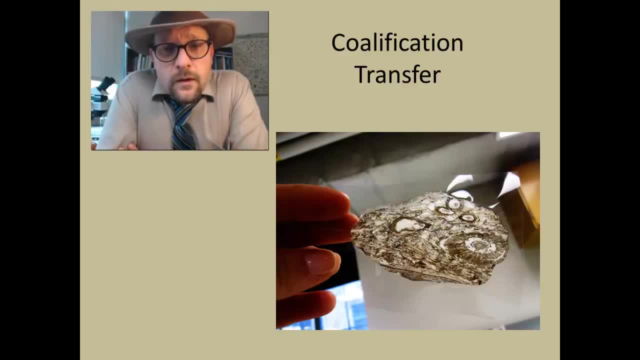 can apply and protect to hold together the organic matter as they dissolve away the calcium carbonate or the silica away from the fossil plant, And so these are transferred over. Sometimes these can be transferred over in serial cross sections of a particular rock and where you get some great preservation. 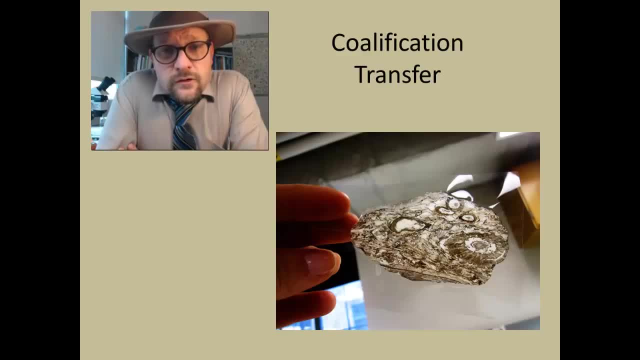 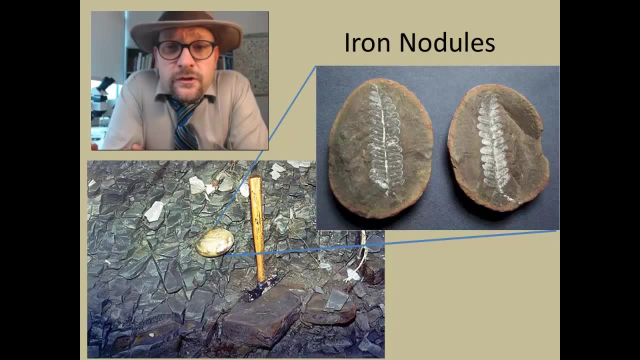 And this is a great way of getting into the detail the internal anatomy of these plants. Another place that fossils- fossil plants- are often found are in concretions- iron concretions. The most famous locality where iron concretions are found are the Mason Creek localities, where 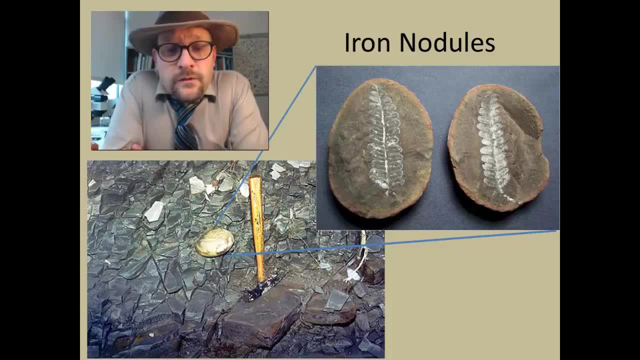 you basically find these concretions, You break them apart and often times you find plant material within these iron concretions. What's interesting is it might be the actual plants that are laid down and get surrounded by these concretions that help to actually form and protect them from the surrounding. 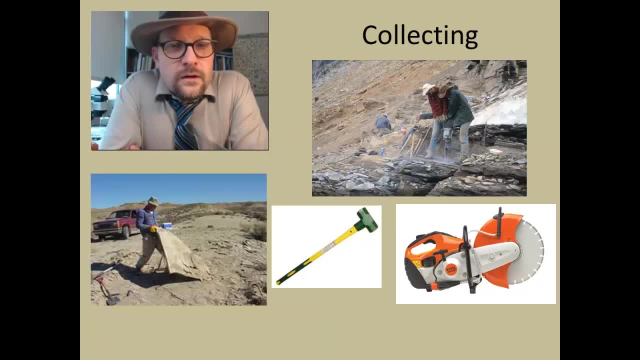 mudstones. Now, collecting fossil plants is a bit different than collecting invertebrates, where, often times, when you're collecting invertebrates, you're just going along the surface and you're looking for anything that's exposed. These fossil plants are made out of this organic matter and so they're very fragile, so if they're 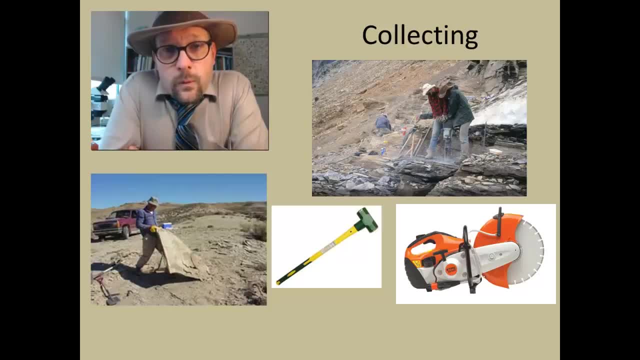 exposed to the surface, they often times will weather away and disappear. So what paleobotanists do in collecting is they go out and they basically try to uncover or peel back various layers or shales and open up and try to get as broad of a surface. 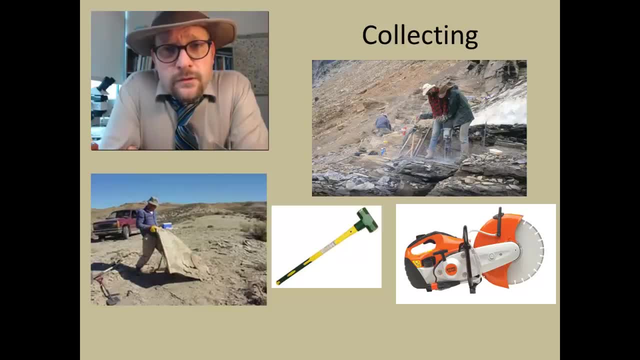 as possible and as they split open those shales and expose that they often will find as they split the shales. So collecting fossil plants is a bit different. the tools of the trade are rock saws, jack hammers and big, huge, giant sledge hammers that are used to break apart these big, huge. 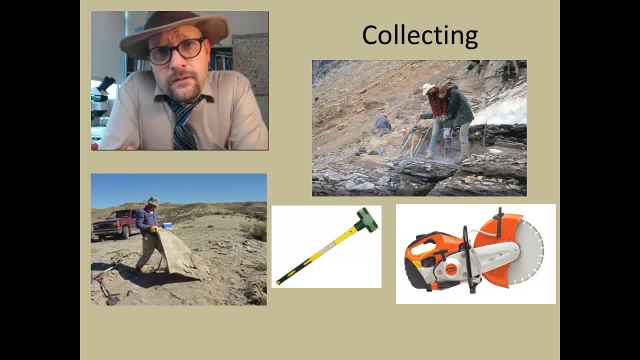 slabs, and the reason you're going for really big slabs is you want to have a nice, preserved, complete specimen, and so if you are breaking apart you know little teeny pieces, the chance of you breaking through one of the leaves or something like that and destroying it are. 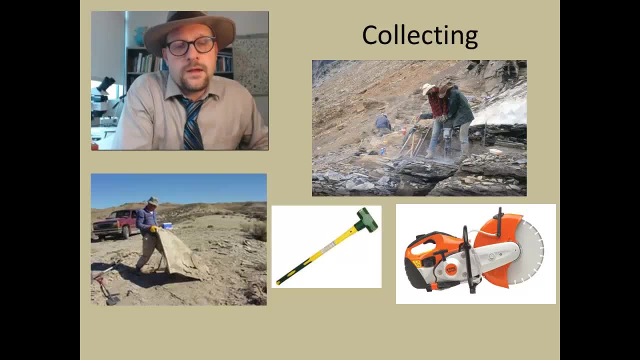 much greater. so the bigger slab you pull up and flip over to look at, the more chance you're going to get a complete specimen, a complete leaf that you can study. So what I thought I would do is go through a little bit about the leaf and wood anatomy. 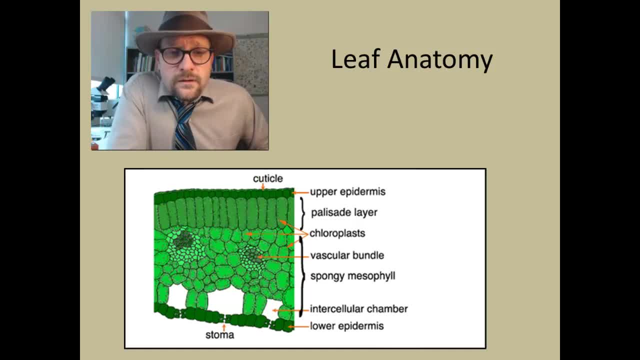 of plants and talk about the various layers. so this is a typical cross section of a typical leaf. On the upper side- so the side that shines to the sun, that gets the most direct sunlight- we have a thin membrane that's called the cuticle, and this is a waterproof membrane. 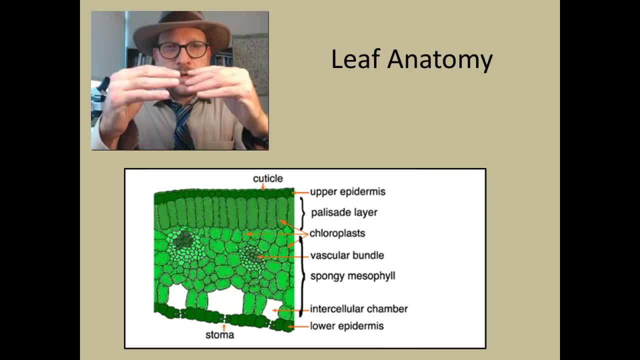 that's on the top and it's basically almost like a waxy surface on top of the leaf, and this prevents water loss, because these leaves are trying to do photosynthesis. they want to be up in the light and often times the sunlight is very high. 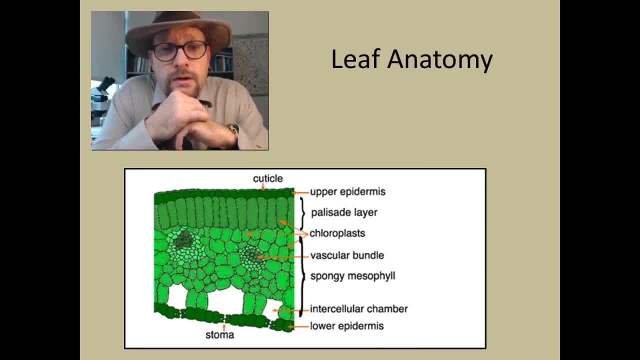 Very hot, and so it dry out the leaf and kill the plant very quickly if it didn't have this cuticle. amazingly, sometimes these cuticles actually preserve in the fossil record, and we'll talk a little bit more about that later on and some of the uses of that cuticle when. 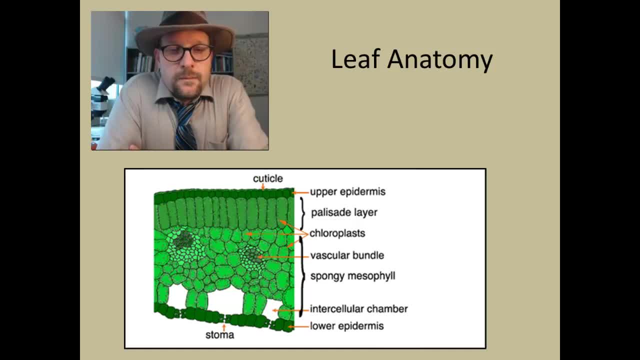 they are preserved. Underneath the cuticle is an upper epididymis, so the kind of outer cell layers, and then we have the palisade layer underneath that and in all these cells underneath we have chloroplasts. I'll talk a little bit more in detail with chloroplasts, because that is the photosynthesizing. 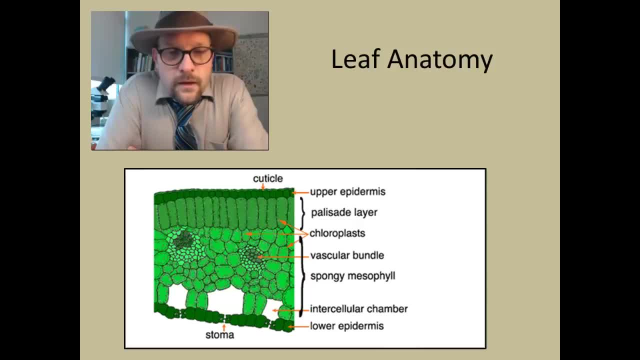 organelles of the cells within plants. In vascular plants you have vascular bundles. these are going to be bundles of cells that help transport water, which is very vital to these cells, as well as transport sugars and various nutrients to other cells that may not necessarily be in that photic zone where 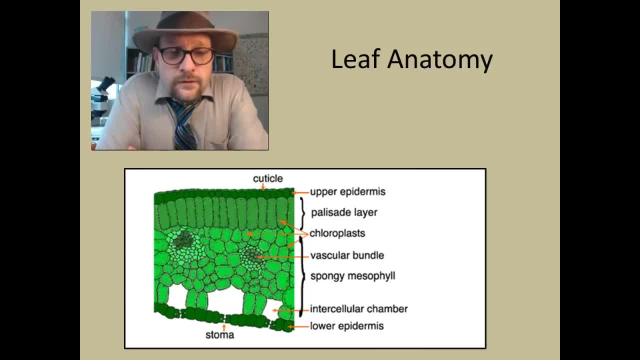 you're getting lots of sunlight And then underneath that You have these sort of these chambers that open up. they have like a door on the underside of the leaf and those doors are called stoma, and the reason you have these chambers and stoma is to get rid of the buildup of oxygen, which is then released through the stoma. 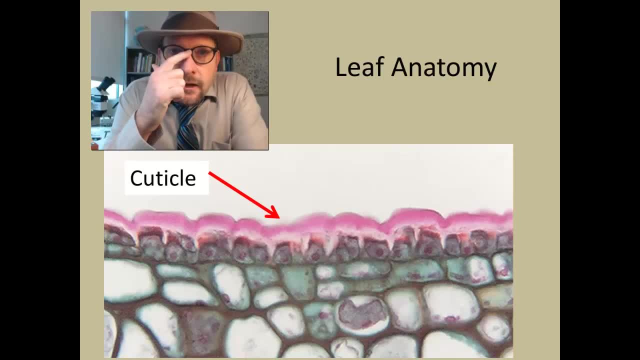 Here's a really nice image of the cuticle. so the cuticle is a second, a cellular. so there's no cells there, it's just basically secreted on the surface of the leaf and so that helps protect. it's a waterproof zone there That helps to protect but is transparent so it allows the sunlight to shine through. 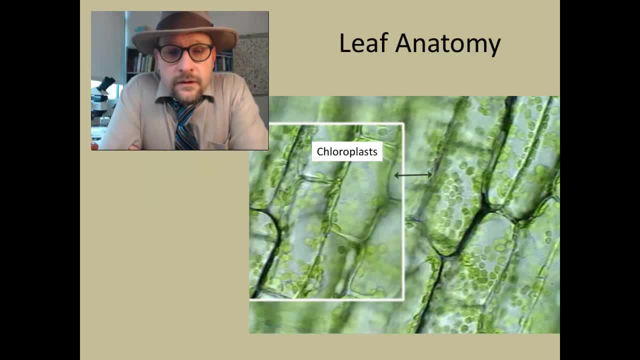 Now, chloroplasts can be seen in all plant cells and in many algae cells we'll talk about later in the next lecture. So chloroplasts are these organelles within the cells that are involved in photosynthesis, and they're often green in color, and this is one of the reasons that plants are green. 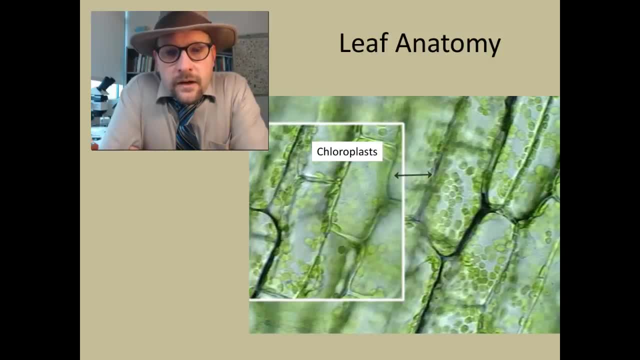 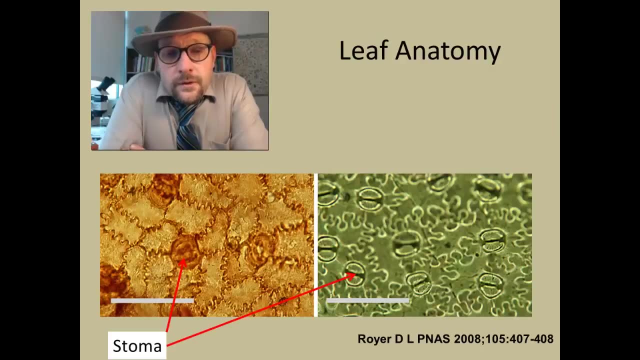 is because their cells are covered in chloroplasts. Chloroplasts, Chloroplasts- organelles which have green, blue and yellow pigments that make green. Now the stoma, the stoma on the bottom part of the plant. these are the doors that open. 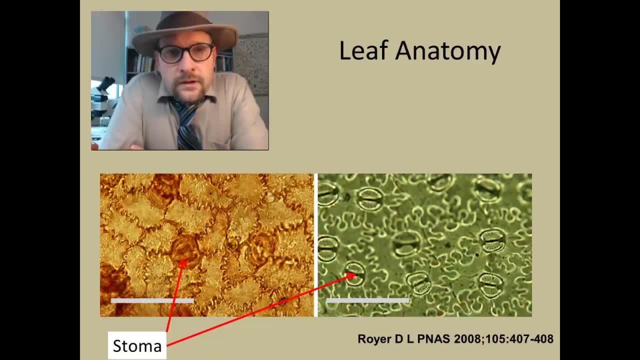 up in many plants. these open up only at night to release the buildup of oxygen, and they do that because in the heat of the day they don't want to lose too much moisture. so many plants rely on water for the process of photosynthesis And they're very 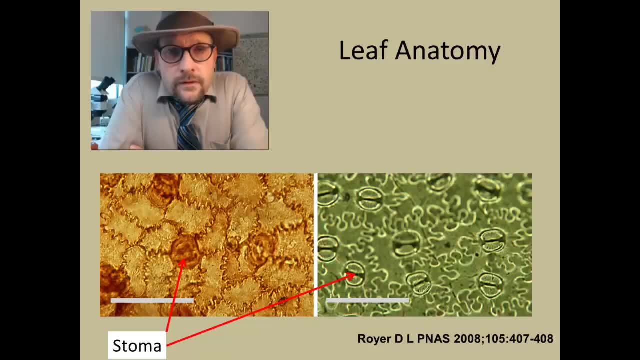 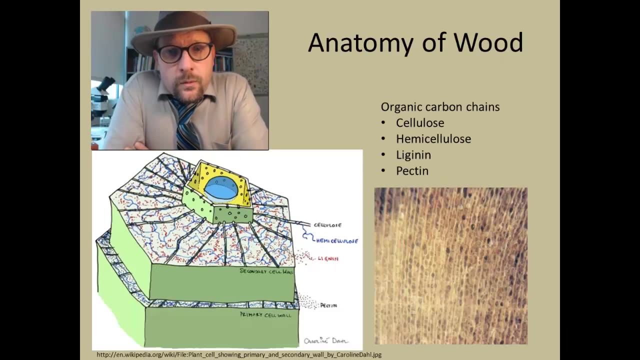 By opening and closing these doors on the bottom part of the leaf- the stoma- they can regulate how much water is lost. These are stoma and you can actually see these under a microscope on the bottom surface of leaves. Now let's talk a little bit about the anatomy of wood and what wood is. 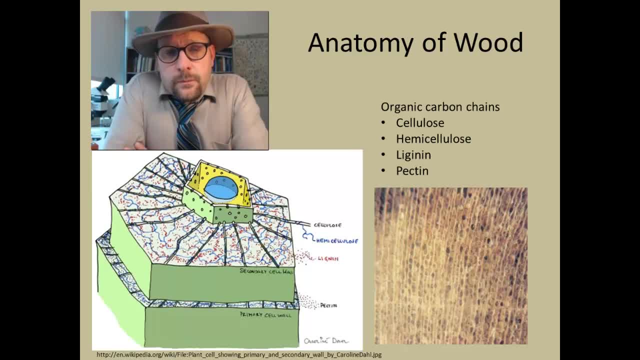 Wood is composed of various organic carbon chains that are bonded to hydrogen and phosphorus and nitrogen, these long polymers of carbon. There's a variety of different ones. The first is the cellulose. Cellulose is these very stiff, fibrous molecules that develop and grow out, and this really 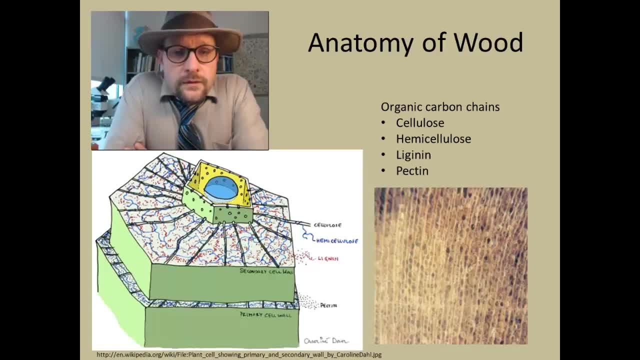 provides the rigid framework of the wood. These are surrounded by hemicellulose, that kind of wrap around and hold the fabric together, and then sprinkled in between these various layers are some polymers, that kind of hold everything together. This includes lignin and pectin. 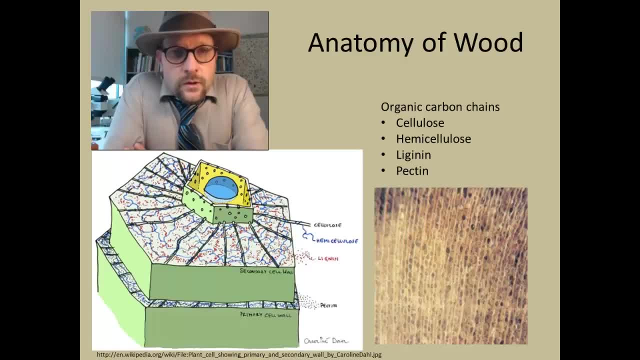 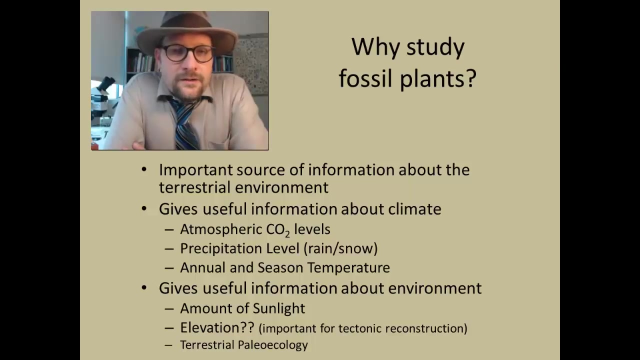 And these basically hold the tissue of the wood together, And then you have vascular bundles where water can flow through capillary pressure through the wood and help to provide water to those leaf structures up in the higher parts of the plant. Alright, so the real purpose of studying paleobotany is that fossil plants tell us a great deal. 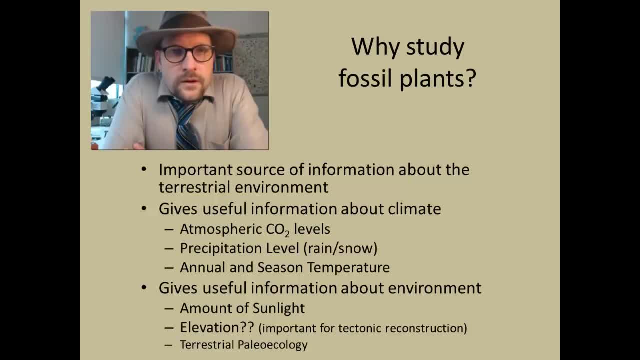 about the ancient terrestrial environment, So they can tell us things about how much atmospheric CO2 was there at particular points in time, how much precipitation, how much rain, how much snow, what the annual and seasonal temperatures were like. Fossil plants give us a proxy for figuring out what the ancient temperatures were like.